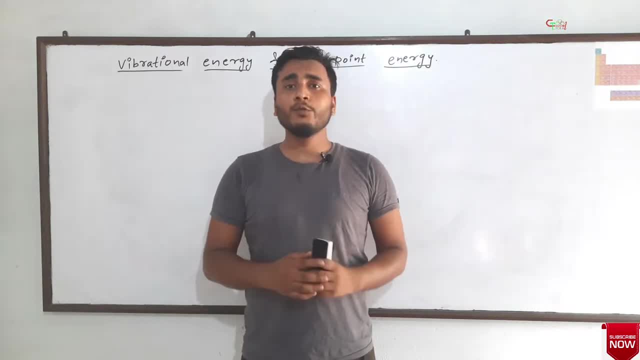 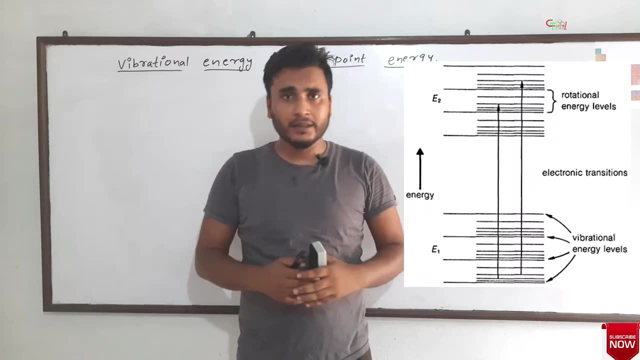 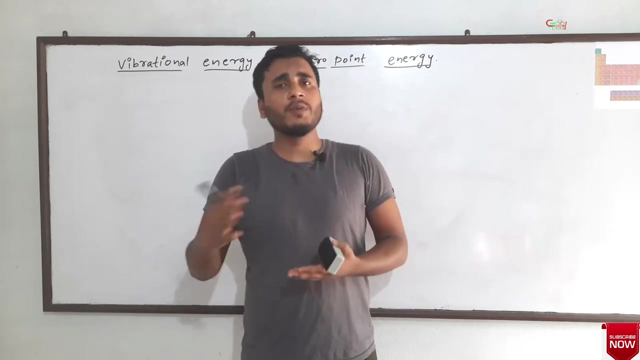 We know that vibrational spectra arises due to the transition between the different vibrational energy levels, and the spacing between the vibrational energy levels is larger than the spacing between the rotational energy level, So more amount of energy has to be supplied to get the vibrational spectra. One more thing: rotational energy was calculated by considering the molecule. 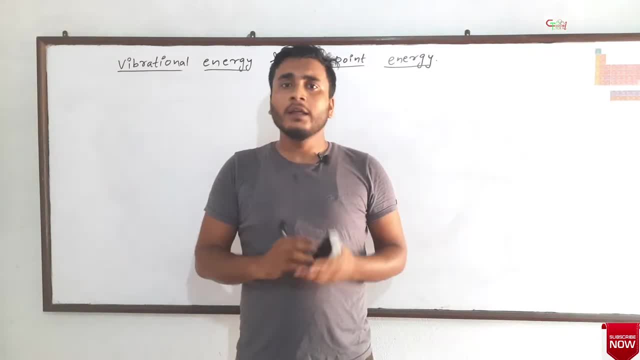 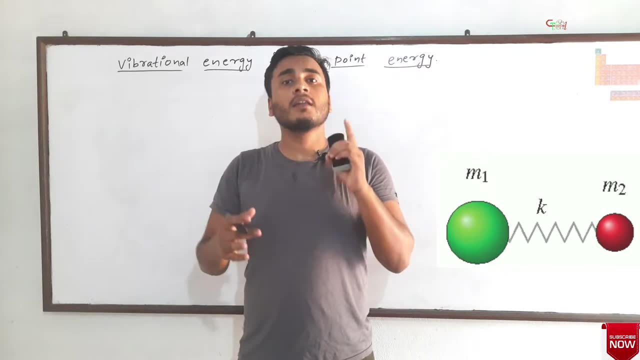 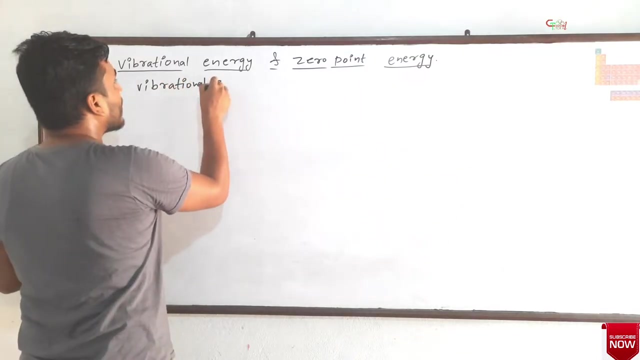 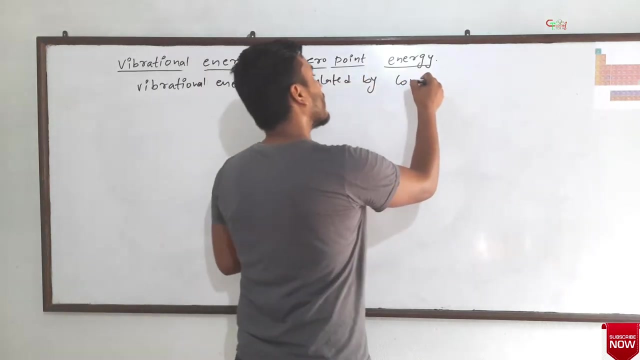 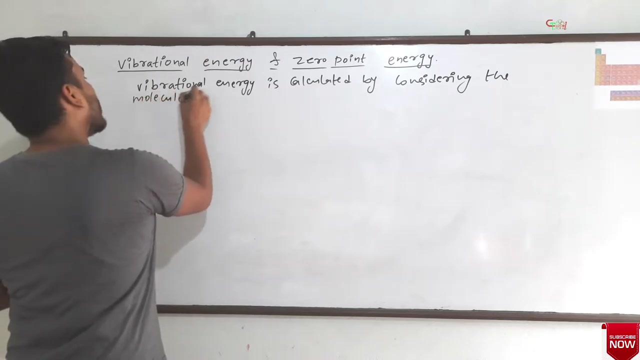 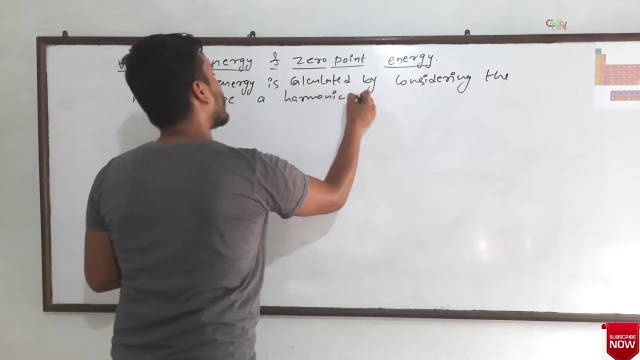 to be rigid rotor. That means they cannot rotate. In the same way, vibrational energy is calculated by considering the molecule as a harmonic oscillator. Okay, so vibrational, vibrational energy is calculated by considering, by considering the molecule, by considering the molecule to be a harmonic oscillator, Harmonic oscillator, Harmonic oscillator simply means they. 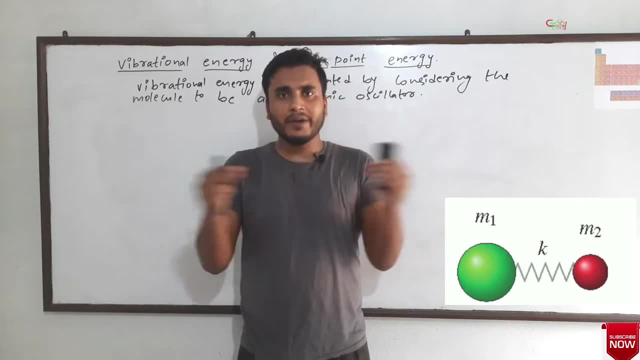 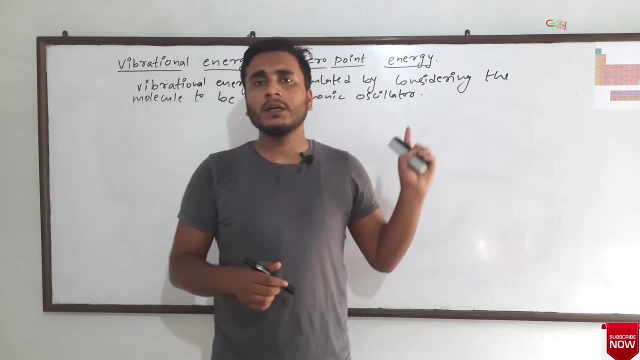 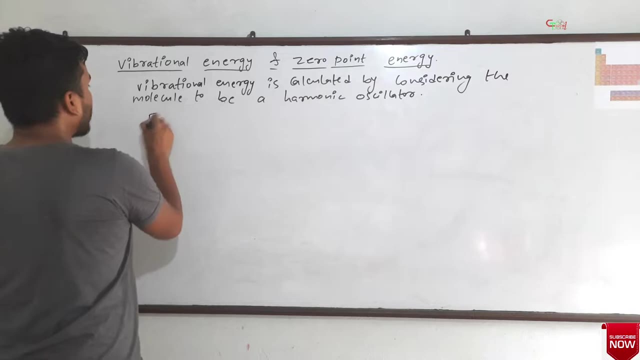 vibrate perpendicularly. Okay, they vibrate perpendicularly like this: Now, by using this condition, we get a formula for the energy of vibrational spectra or vibrational level. Okay, that formula is therefore EV. EV means vibrational energy is equal to. it is equal to h, nu naught v plus 1 by 2.. So this is the formula for. 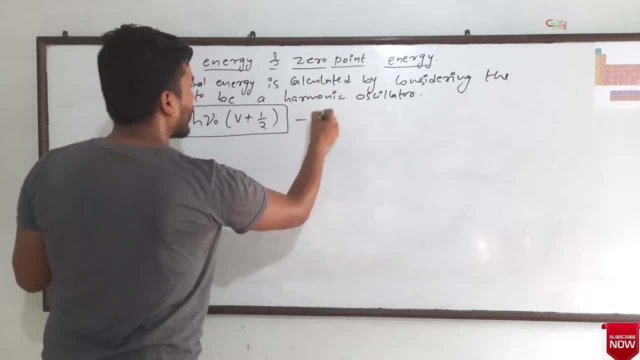 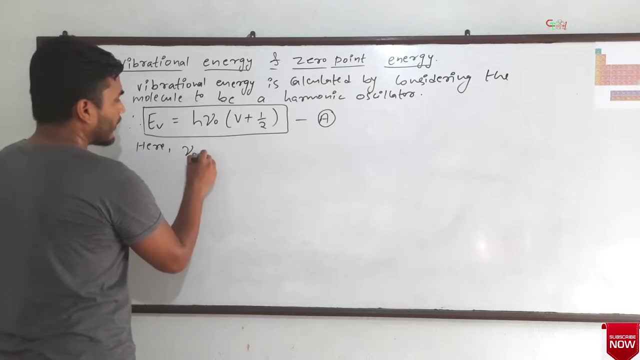 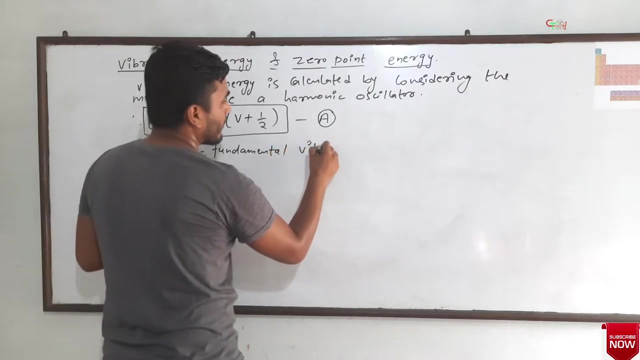 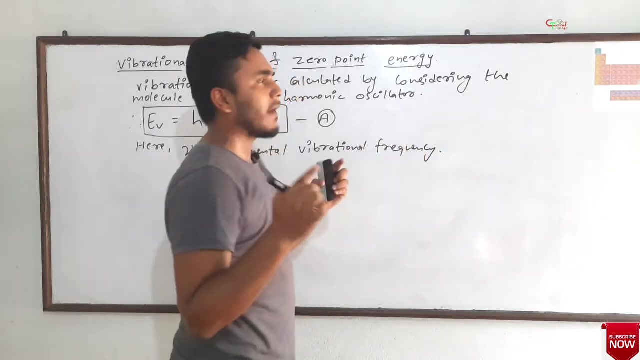 the vibrational energy. Let's consider to be question number A. Okay, here, here, this nu naught, nu naught is fundamental, fundamental: vibrational frequency. vibrational frequency: We know that if the molecule vibrates, it must have certain frequency. we 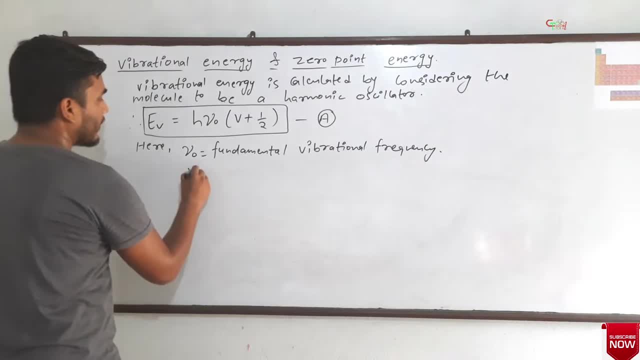 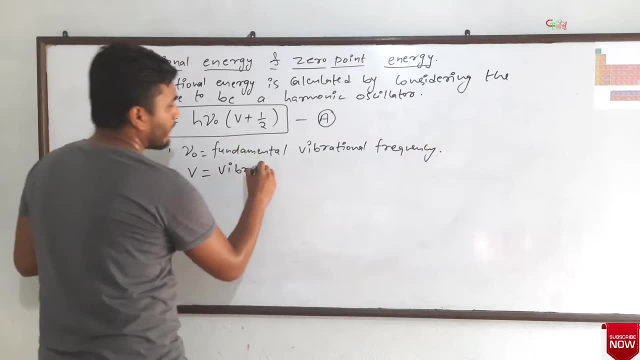 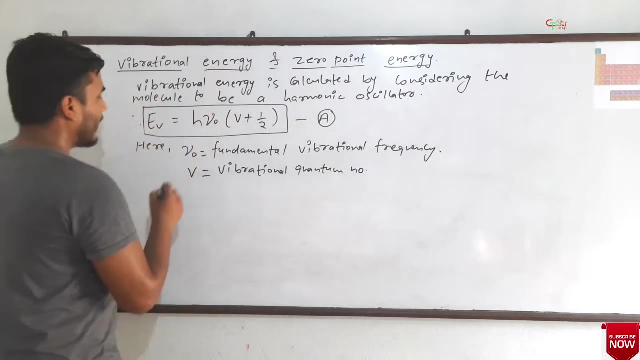 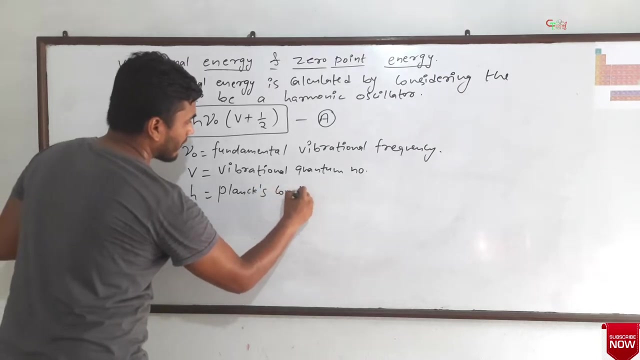 have considered it to be nu naught V. V means vibrational, That is, this V, Okay, This V, This V, Vibrational quantum number, Quantum number, And this H means, you all know that, Planck's constant, Planck's constant. 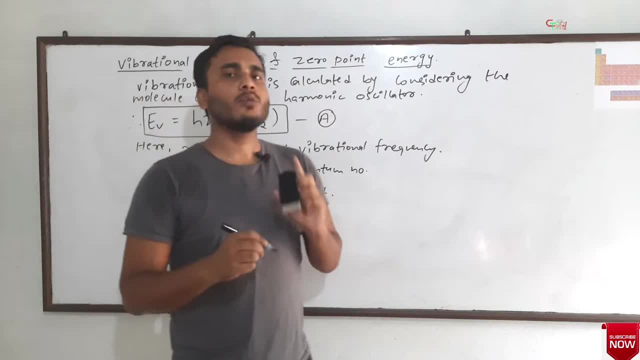 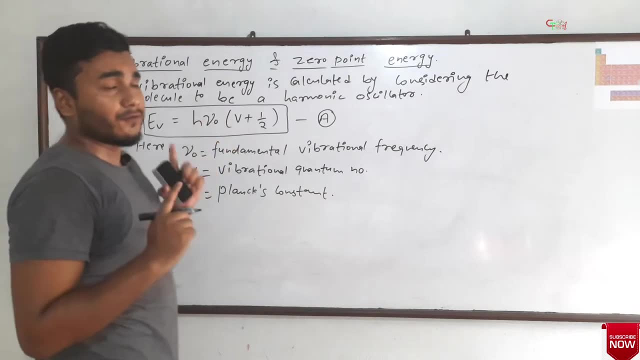 So this is the formula by which we can calculate the energy of vibrational level. You can see over here, If we put the value of V to be 1.. As V is the quantum number, That is, V can be equal to 0,. 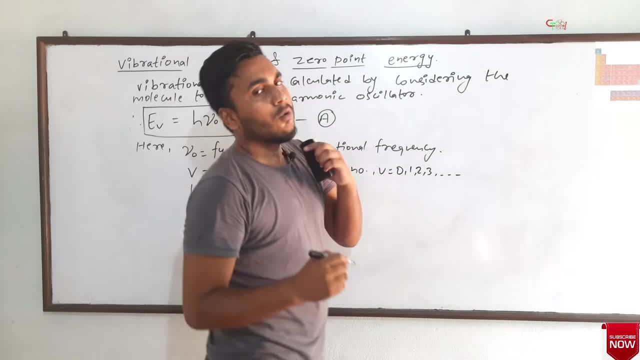 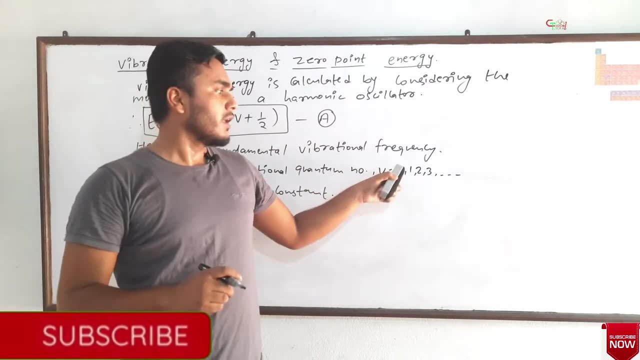 1,, 2,, 3.. Just like rotational quantum number- We denoted rotational quantum number by J- We denote vibrational quantum number by V. Its value starts from 0 and it keeps on increasing with different vibrational energy level. 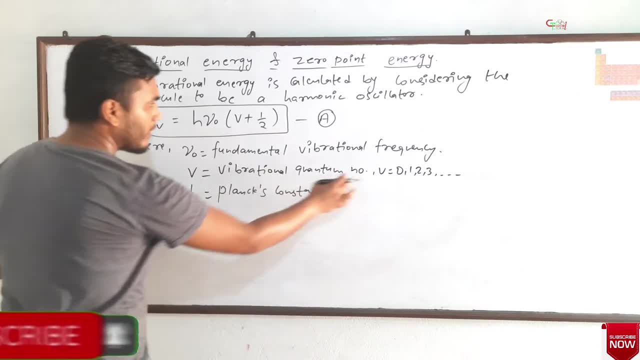 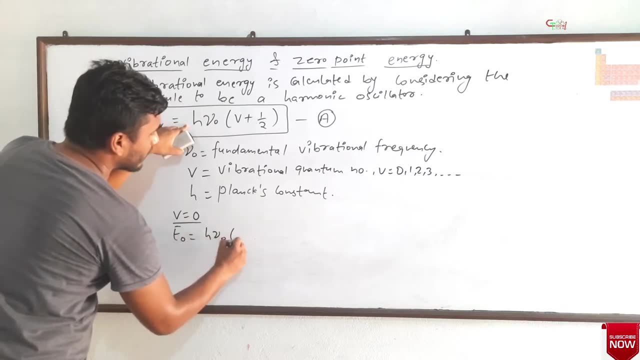 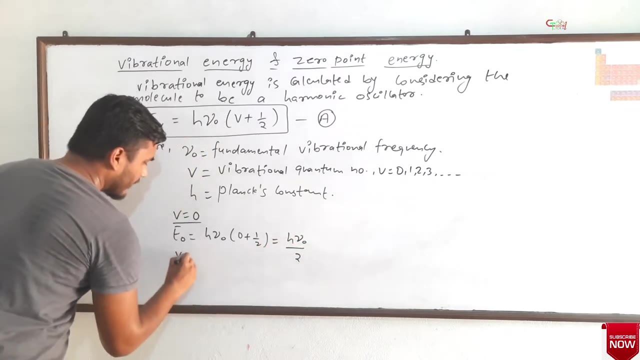 Now when V is equal to 0. If V is equal to 0, then what do we get? E0 is equal to E0 is equal to H nu naught 0 plus 1 by 2. It simply means H nu naught by 2.. If V is equal to 1, then we get. 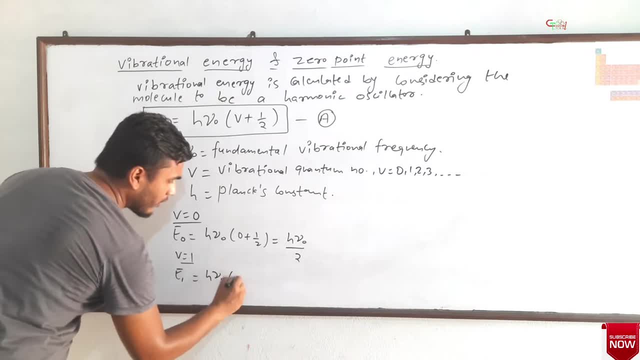 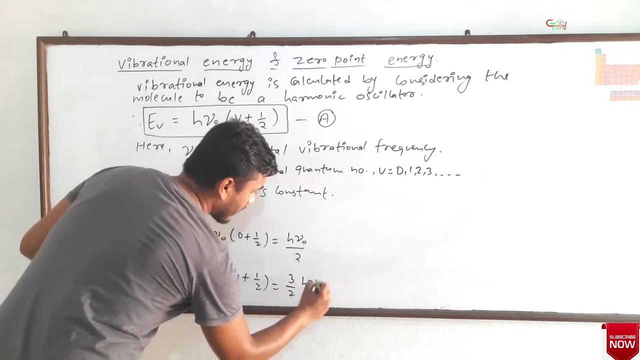 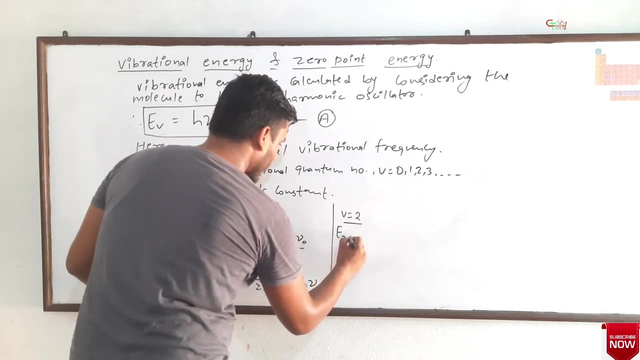 E1 is equal to H nu naught, 1 plus 1 by 2.. If we add it, we will get how much 3 by 2.. 3 by 2. H nu naught. In the same way, if we consider V is equal to 2, then we will get E2 is equal to. 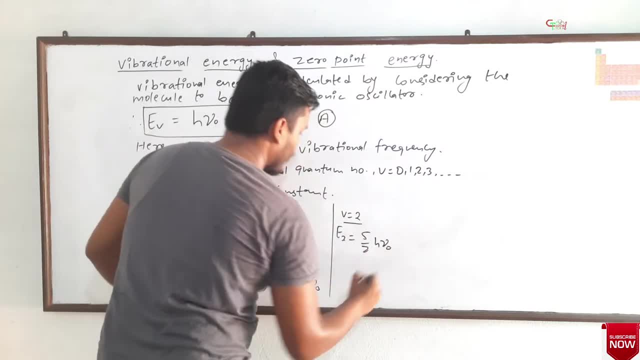 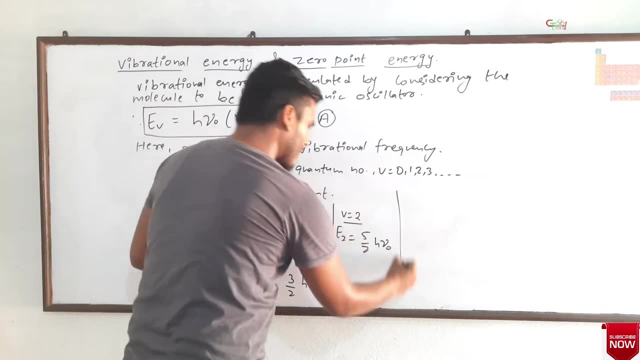 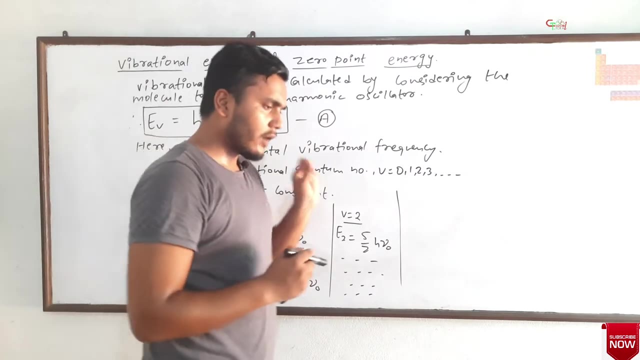 5 by 2. H nu naught. You can easily calculate by putting the value of V is equal to 2. over here You will get this much. Now, in the same way, this value keeps on increasing as we increase the value of V. Right Now we need to see one more thing. A very interesting thing is observed over here. 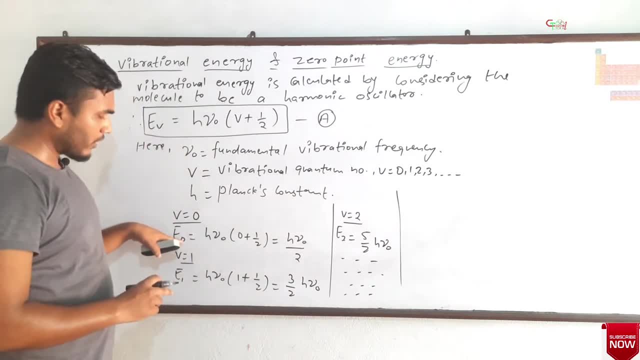 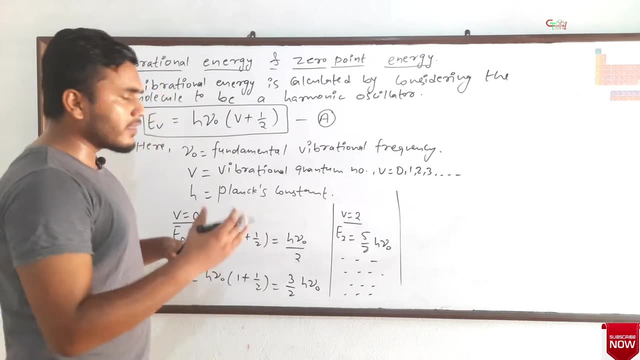 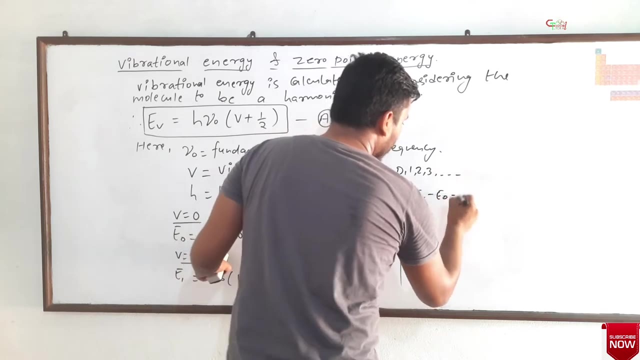 Like: See the See the value. When we put V is equal to 0, then V is equal to 1.. V is equal to 2.. Okay, It has the spacing of H. nu naught That means E1 minus E0.. If we subtract E1 minus E0.. If we do, 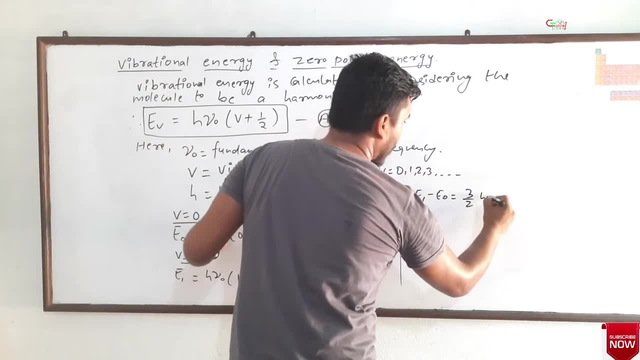 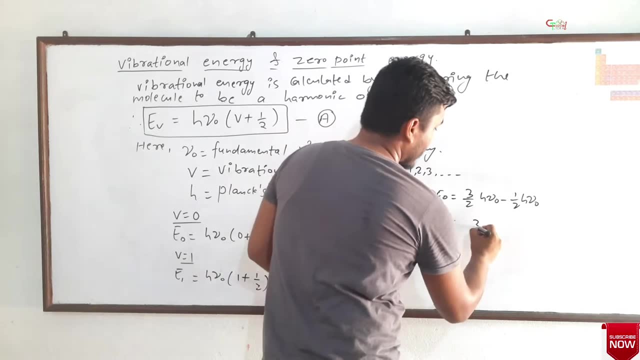 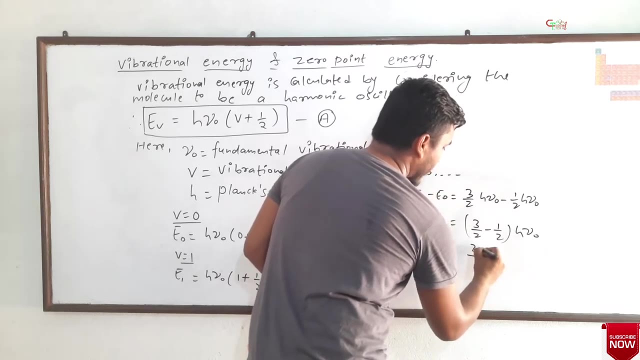 E1 minus E0.. How much do we get? 3 by 2 H nu naught minus 1 by 2 H nu naught? So it will simply be: how much 3 by 2 minus 1 by 2 H nu naught? This is a like fraction, So we can simply subtract it like this: 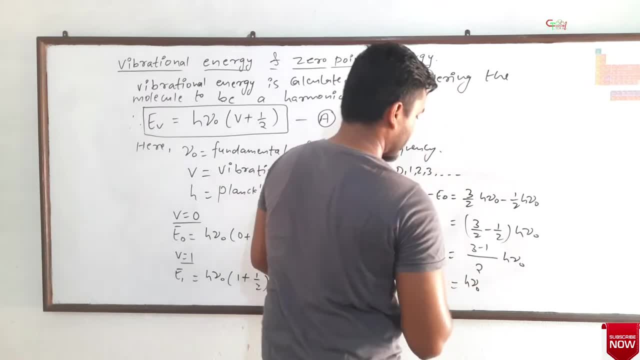 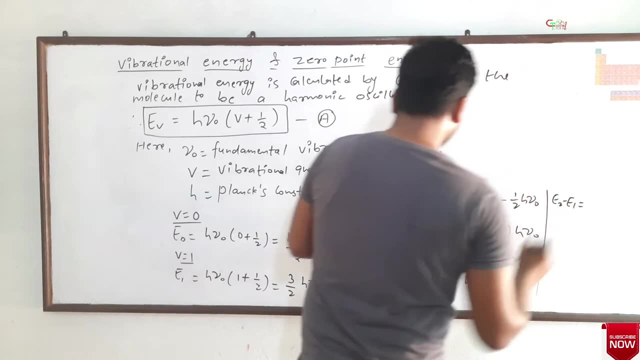 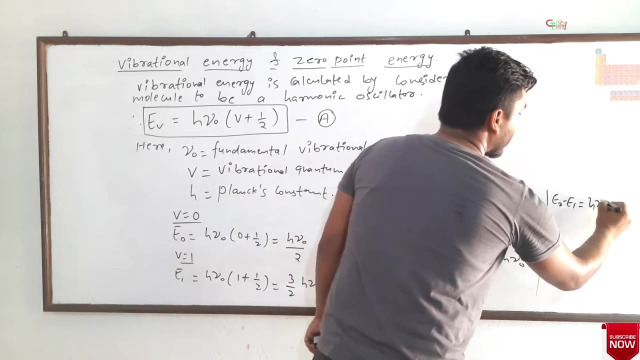 H nu naught, It is equal to H nu naught. In the same way, if we calculate, If we calculate E2 minus E1. If we subtract E1 from E2.. If we do E2 minus E1. Then also we will get how much H nu naught. 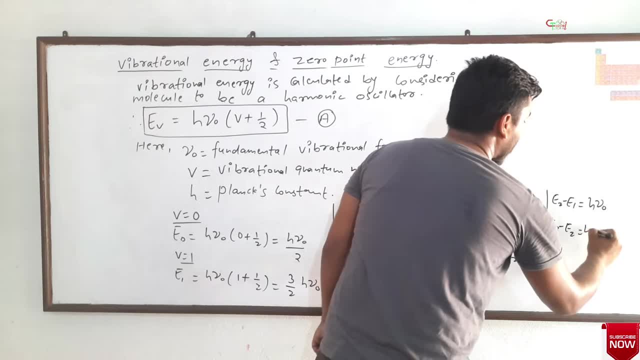 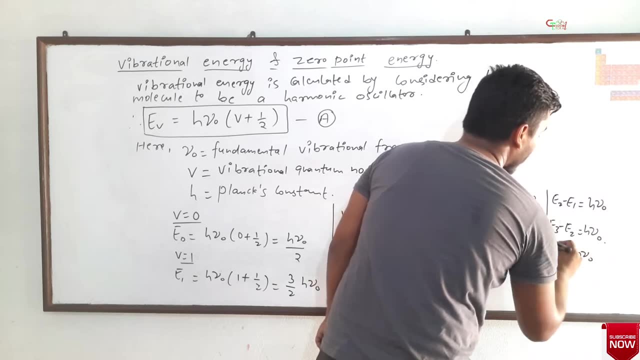 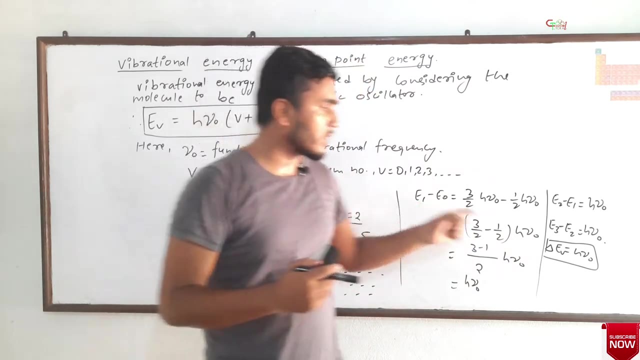 If we do E3 minus E2.. We will get H nu naught. That means del, E will always be Del, VEB will always be how much H nu naught. That means the spacing of the vibrational energy level will always be equal to how much. 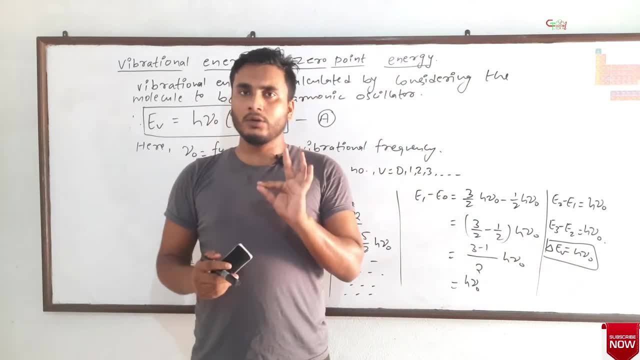 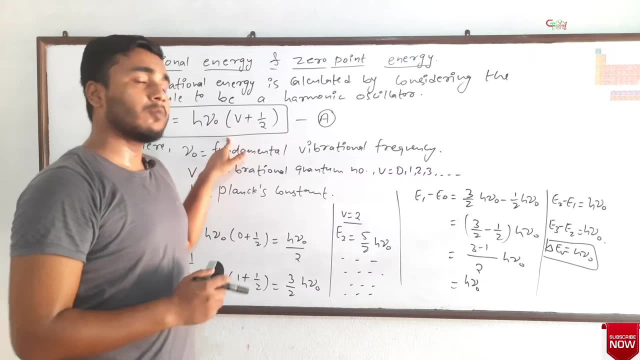 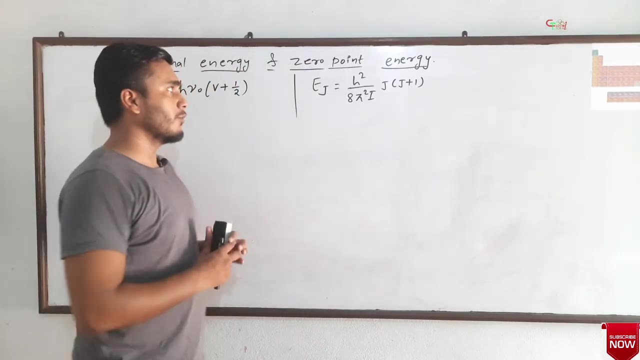 H nu naught, It is constant. Okay, Now, this was for the vibrational energy. You need to remember this formula. This formula is very important. Okay, Now we need to see what is zero point energy. You can see two formulas on the board. The first formula is for vibrational energy level And the 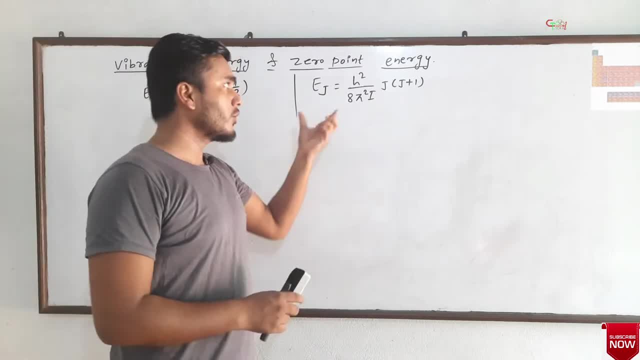 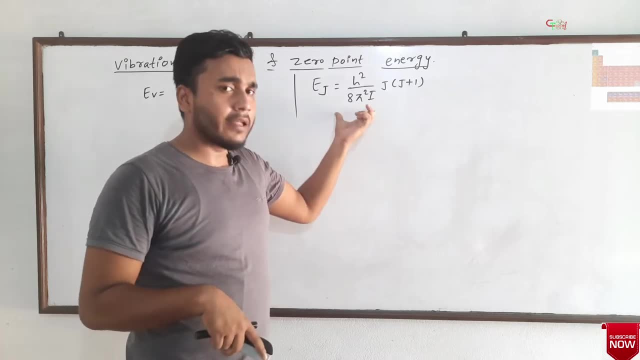 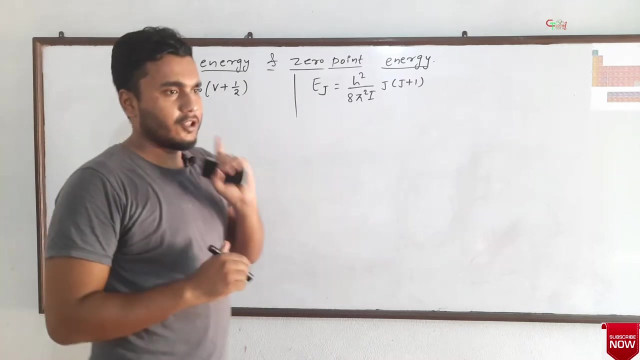 second formula is for rotational energy level. If you don't know how this formula came, Then you can check. in the description below You can find a video. Just watch that video, You will definitely know how this formula came. Okay, Now we need to talk about zero point energy. Zero point energy. 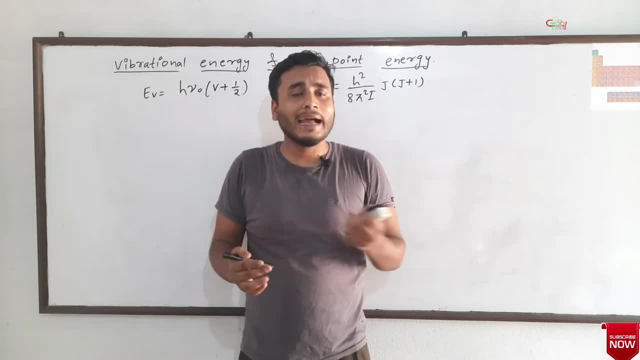 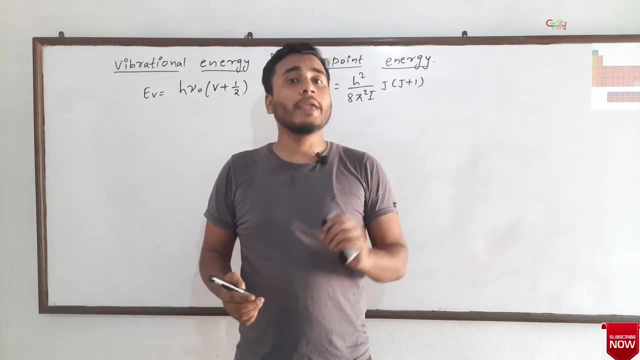 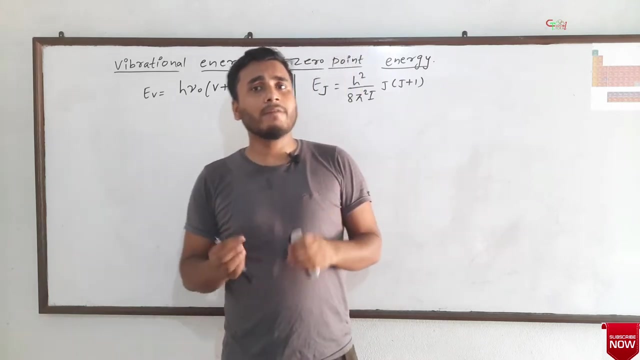 means simply saying what will be the energy at absolute zero of 10 to the power of 0.. So this is the temperature. Absolute zero means the lowest possible temperature, That is, zero kelvin, Right Zero kelvin. Now, at that temperature, the value of rotational quantum number and vibrational quantum. 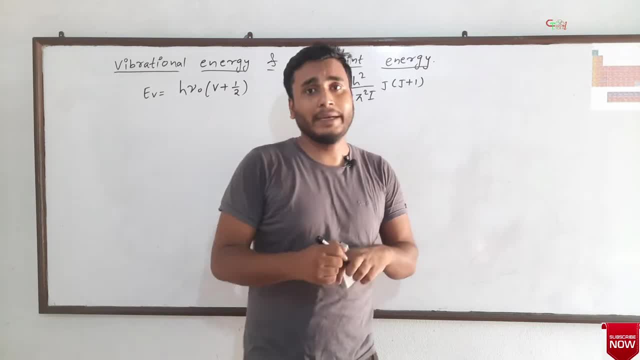 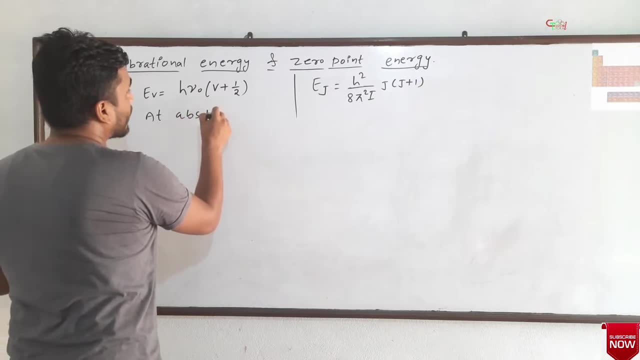 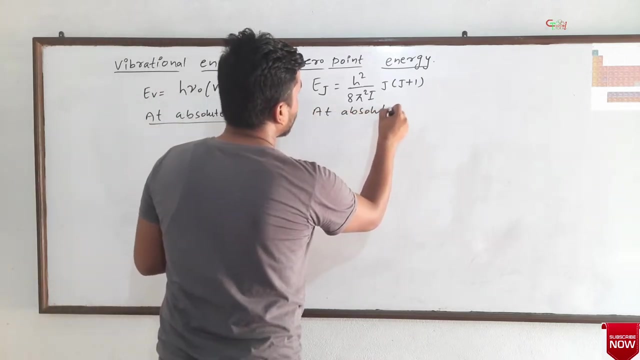 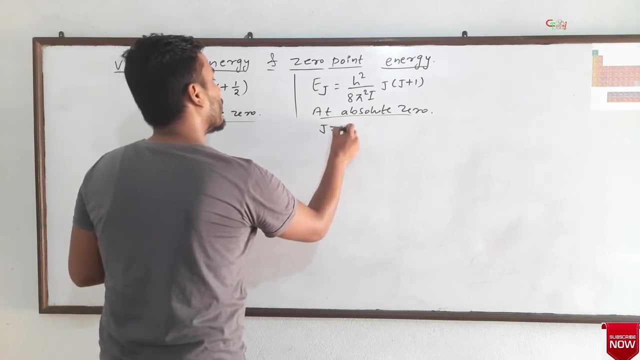 number will be zero. So let's see what happens mathematically. Okay Now, at absolute zero, At absolute zero. Here also, let's write the same thing. At absolute Zero, V will be equal to zero. Here, j will be equal to zero. Then it will be: e is equal to h, nu not. 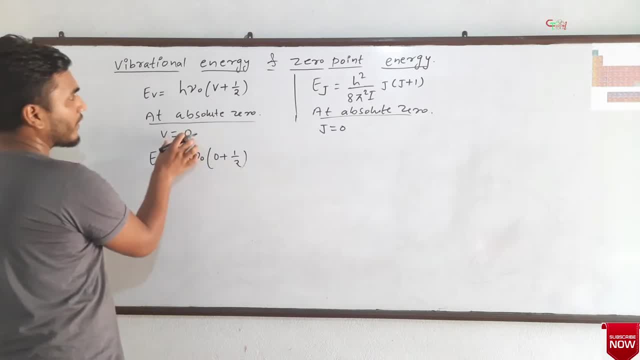 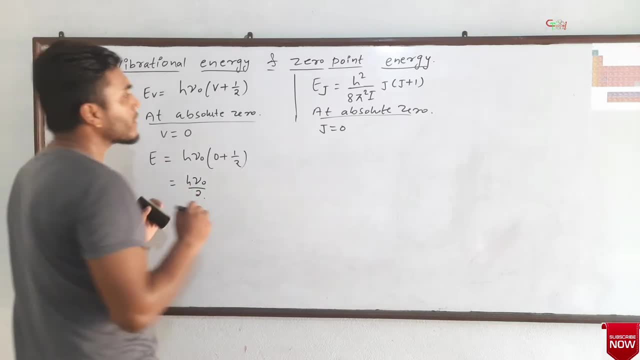 zero plus 1 by 2.. That means in place of v we need to write zero, So it will be h nu, not by 2.. Right, We get this much of value. And here, if we put j is equal to zero, Then how much will we get? 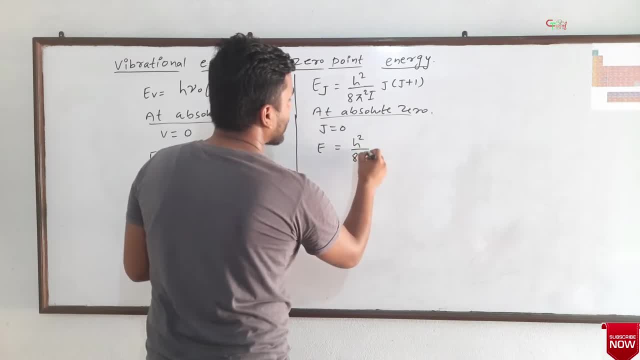 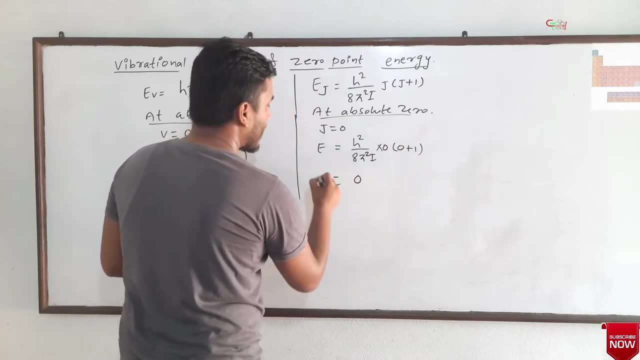 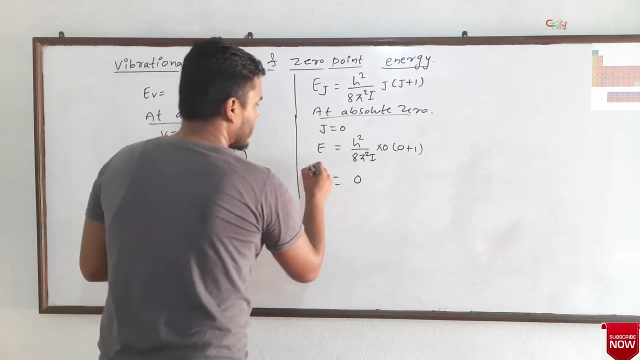 h square by 8, pi square i into 0 and 0 plus 1.. So this zero will make all the value zero. That means e j will be equal to zero And e v will be equal to this much. What do you see from here? 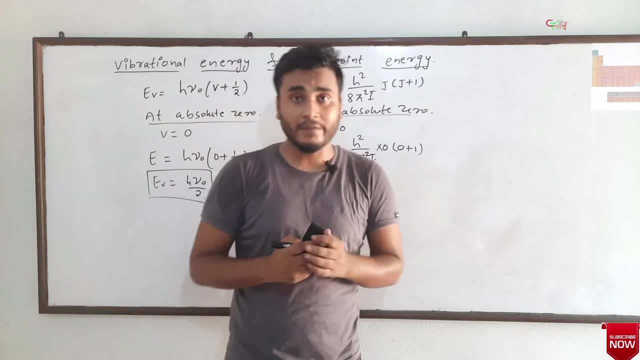 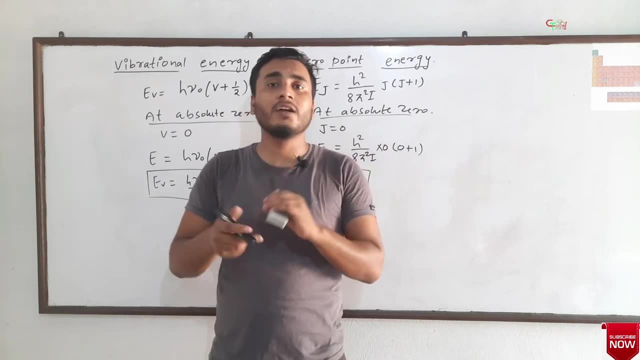 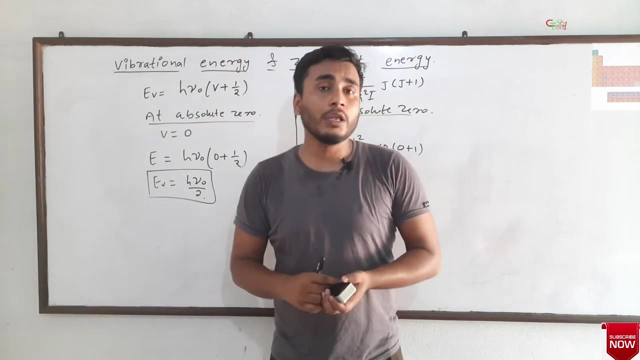 What do you see from here? What is the conclusion of getting this much of value? That means at absolute zero there won't be any rotational energy in the molecule. That means the molecule cannot rotate. But here we are getting certain value. That means even at absolute zero the molecule is not at. 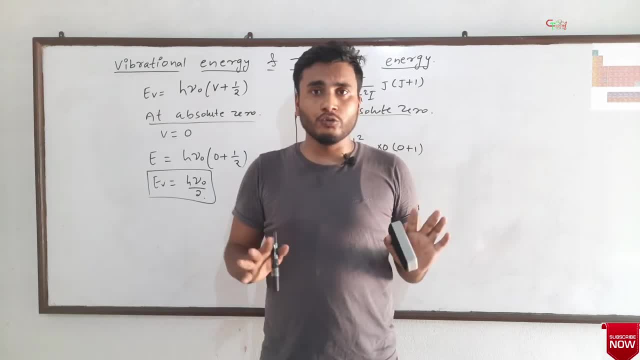 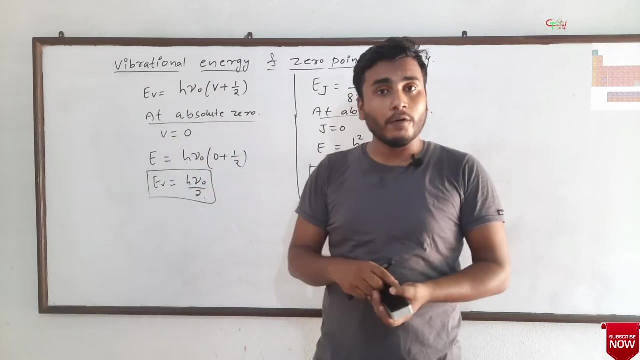 complete rest. It will not rotate, Yeah, That is true, But it will vibrate in perpendicular axis. Okay, Even at absolute zero. molecules vibrate because they possess certain vibrational energy, even at absolute zero of temperature. So the energy, this much of energy, Okay, This much of energy. 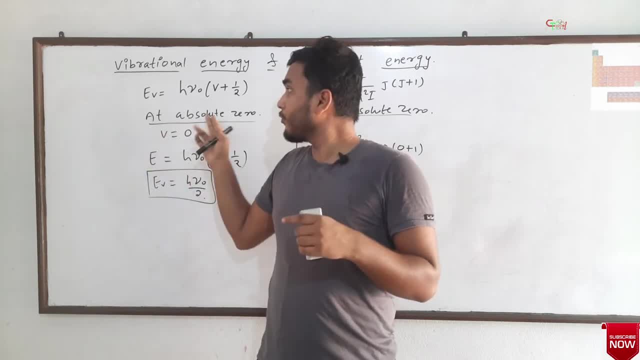 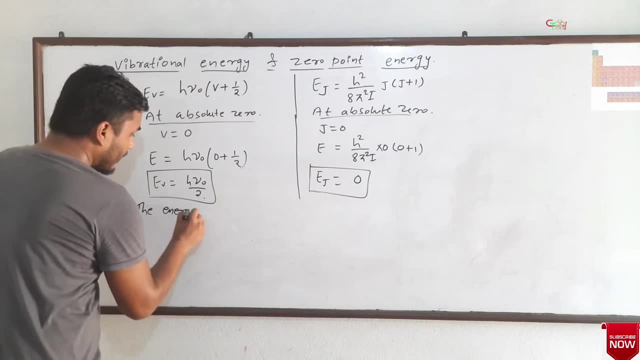 is assigned at absolute zero of temperature as well. So the energy, the energy. let us closer the vibrational energy. The vibrational energy at a absolute 0 is called 0.0 SP بت beep energy. Okay, Very good, Very good. 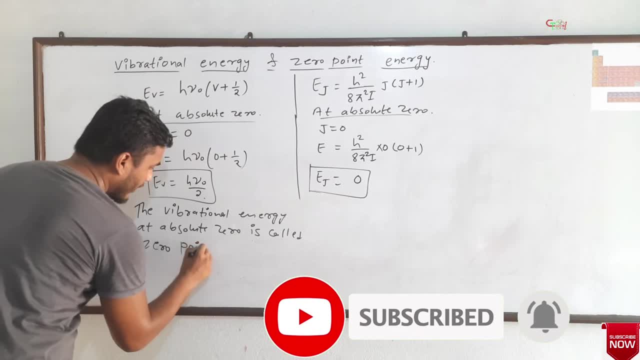 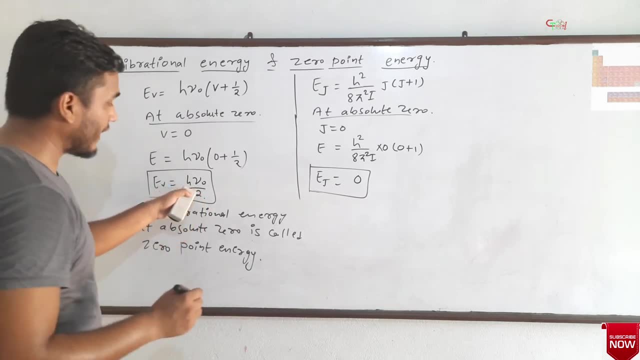 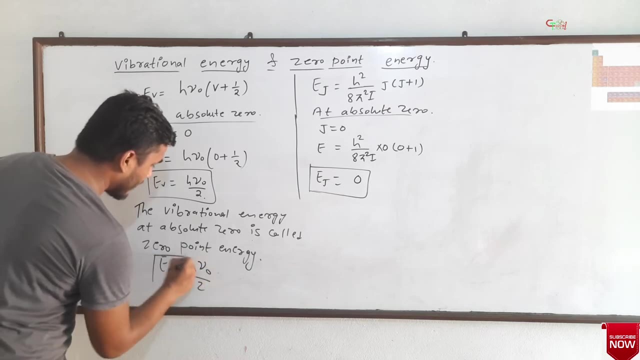 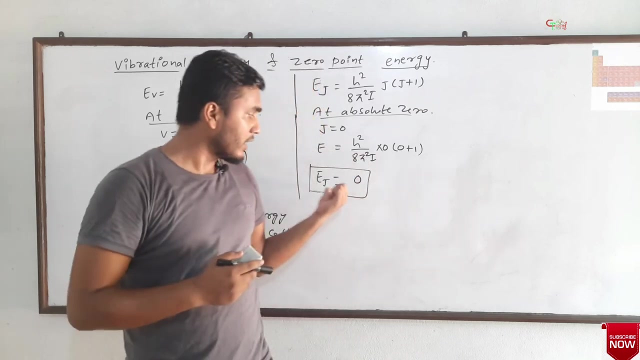 energy is called zero point energy. so this is the value for that zero point energy. okay, this is the value for that zero point energy. let me repeat one more time: at absolute zero, there is no rotational energy in the molecule. that's why EJ becomes zero. that means it cannot rotate now. but even at absolute 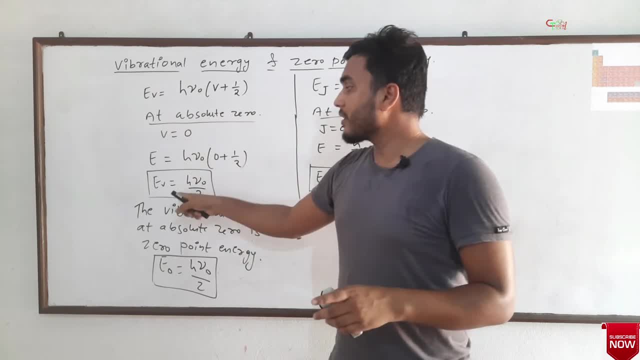 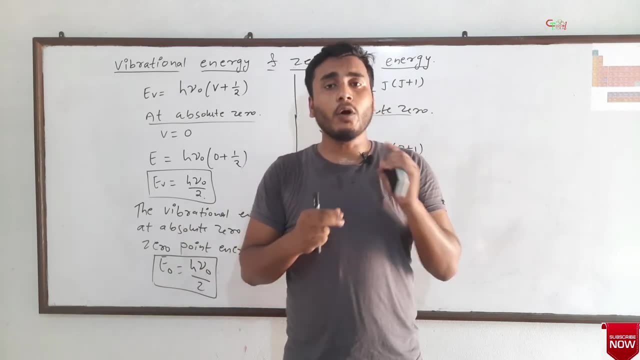 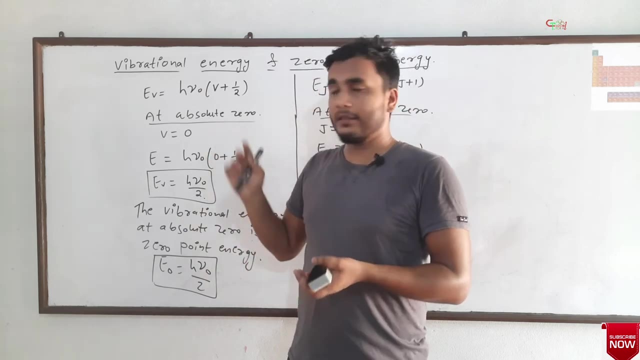 zero, there will be certain vibrational energy. that means this much of value as nu naught by two. that means even at absolute zero they vibrate. so all the molecules will always vibrate, even at absolute zero of temperature. this formula tells that. so this is the value for zero point energy and this is the